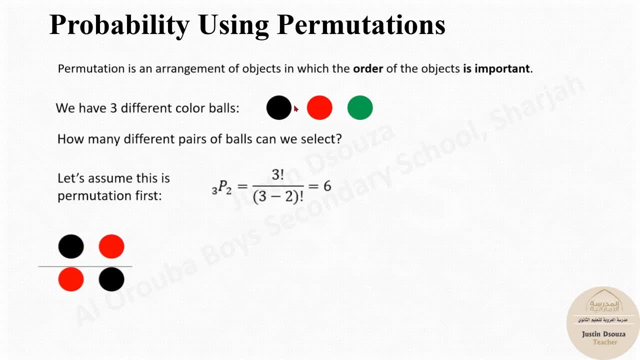 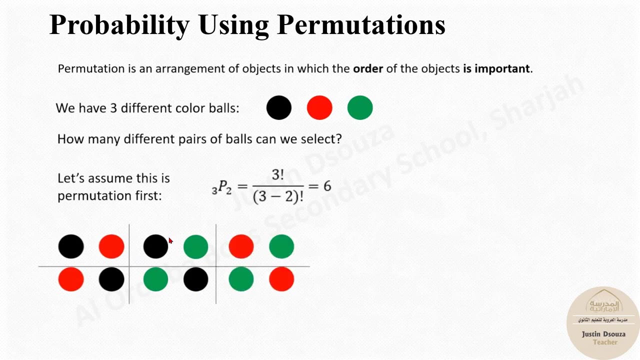 into a look into better understanding. See, there's one way you can select these two: black and red, or red and black. Which order matters here? There are different arrangements altogether. Or you can take, say, black and green, green and black, or red and green, green and red. So these are the six different ways. 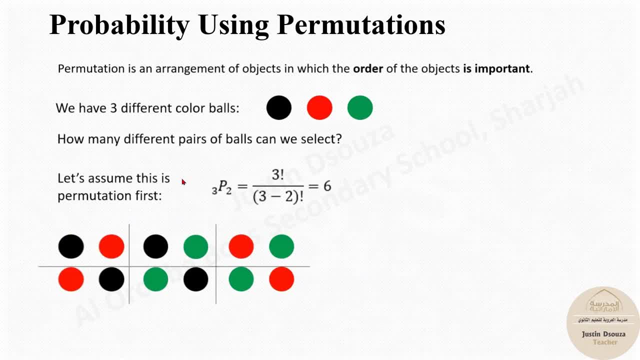 right Now. this was a simple one because we're just taking pairs, But what if the- you know- sample space is huge, in the sense there may be 20 balls and we are taking three at a time. It's going to be a lot of possibilities, isn't it? We can formulate this by a simple formula. 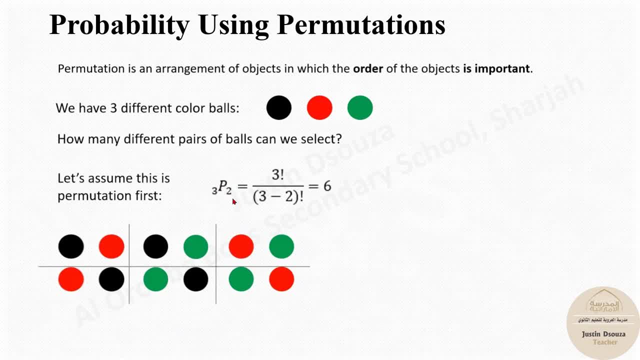 npr or 3p2, which is given by this formula, we are 3 factorial by 3 minus 2, whole factorial equals 6.. Now I will show you how to exactly do that. Now, before we go ahead, let's look into factorials. 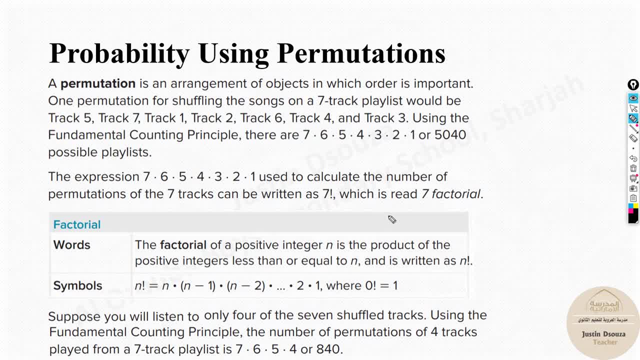 Now, why this factorial is used is because of the fundamental counting principle We had seen in the previous lessons. how do we find all the possibilities is multiply all of them right Now. over here they have given example of different music tracks. okay, there are. 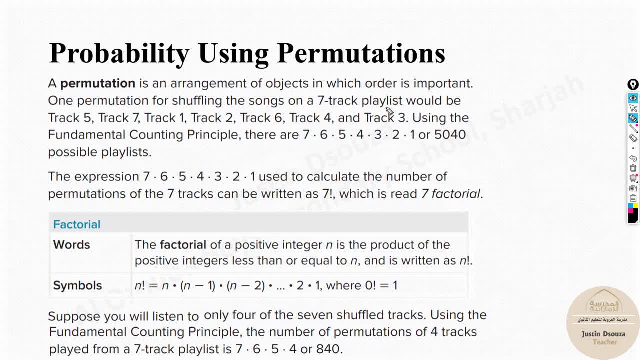 seven playlists, seven track playlists. now, what are the all possible ways to select them? now, when you select them, the first possibility would be all seven. you can select anyone. all seven, but then, once this is done, how many remains? six for the second song, and five and four and three and so on. right instead of all. 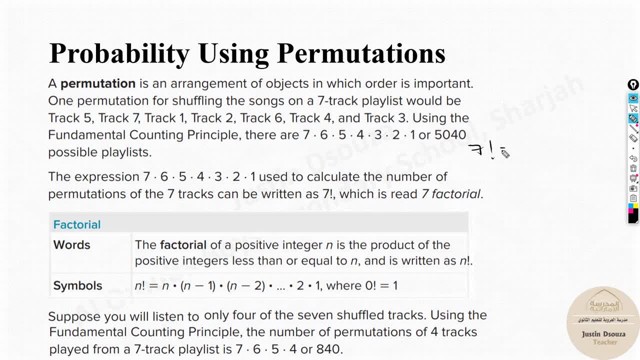 that what we will do is we'll consider it to be seven factorial. this means first you multiply this number seven and then one less than that, it goes n minus one, that's six multiplied by n minus two. now n is this seven, n minus one is six. 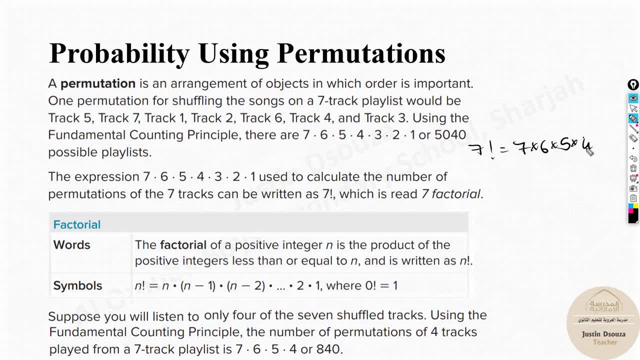 n minus two is five, and so on until you reach one. okay, you don't multiply with zero when you reach one. that's the thing. and if you're thinking, what is zero factorial? it is equal to one as well. okay, so factorial is an easy way to solve these problems. and now, if you're 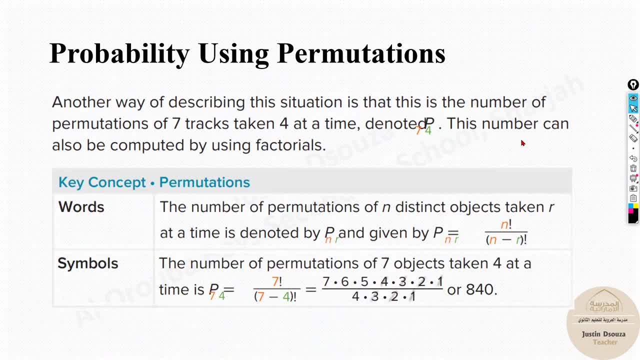 thinking about the formula of NPR which we saw just a while ago. this is the formula here: NPR. see, there's various ways to write it. now. one way is N over here, and then P caps. P are like this, for some right NPR, or they write it down. 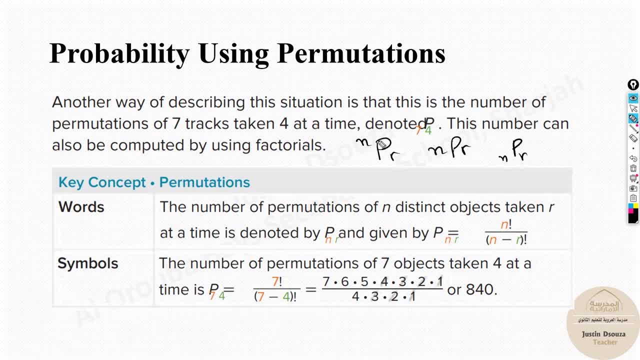 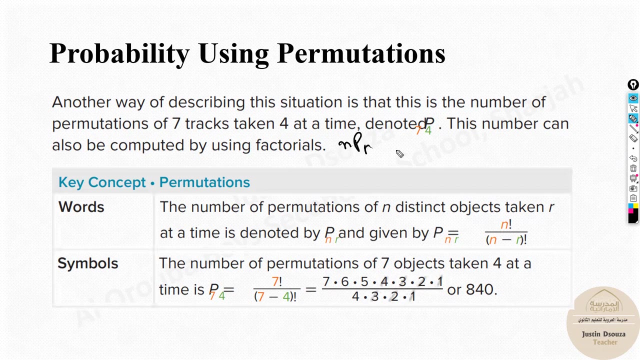 NPR. you can write superscripts: letter subscript, subscript, normal, just letters and small letters, or subscript subscript. subscript means anything that is down here, superscript is something that's up above. now then let's see. if you have see, this is the formula, let me write it: NPR. then we need to start with N factorial divided by N minus R. 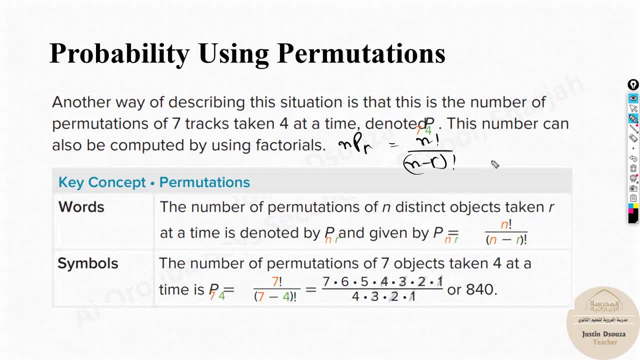 factorial. whenever we use this formula and whatever the answer we get here, the order makes a difference. order is important. so this is the NPR permutation formula and now, if you have any numbers over here, you can see seven and four. the N will be more than R generally, because most of the 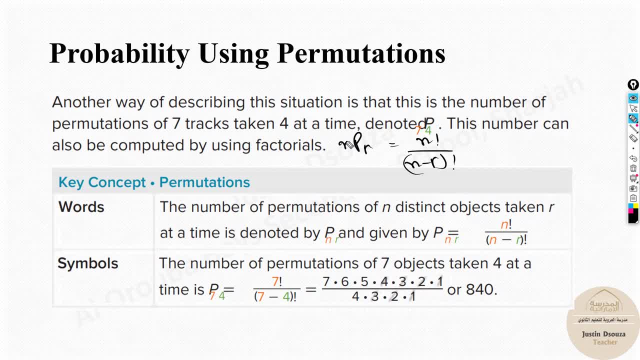 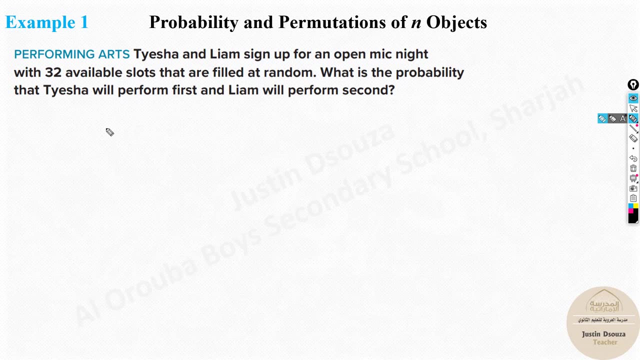 problems. N is the total possibility- total number given to you in a problem will be more clear- and R is the selection. so you just put in this formula and you get the answer. now we'll jump into a problem and apply it. before we start this problem, let us remember what is probability- probability of any. 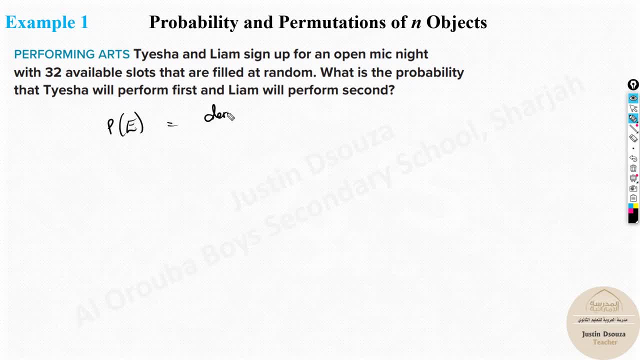 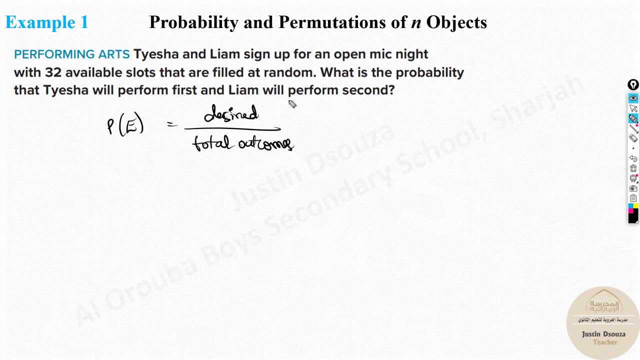 event, it's always the desired, desired outcomes divided by the total outcomes. I hope you remember this. total outcomes now, desire is what you want, what happens, which is the favorable outcome, or what you really want to happen. this is all the total possibilities. the permutation is basically the total outcomes: total. 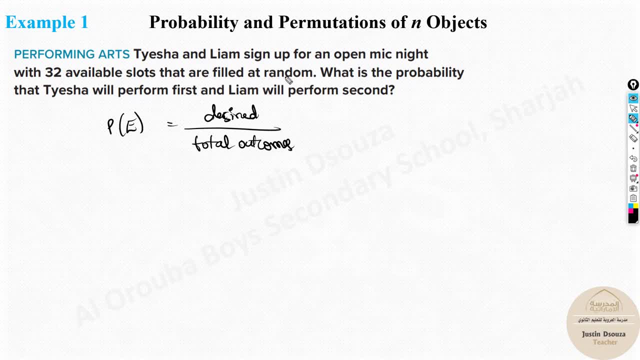 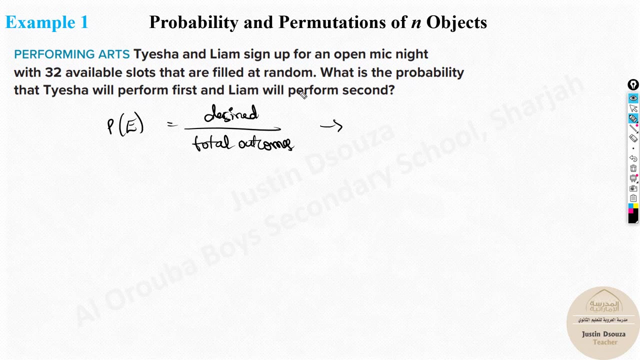 possibility. desired one. desired one is what you need to read the question and understand, and write it out. let's read this question now. taisha and liam sign up for an open mic night with 32 available slots that are filled at random. what is the probability that taisha will perform first and liam will? 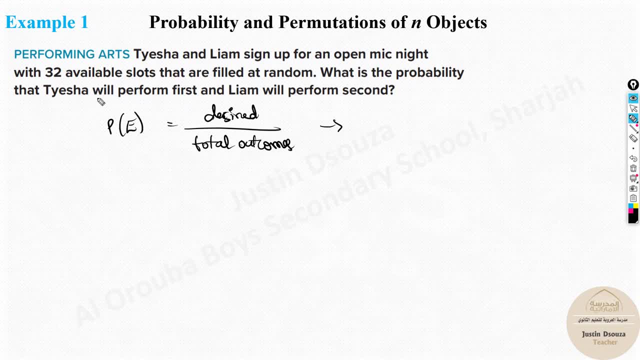 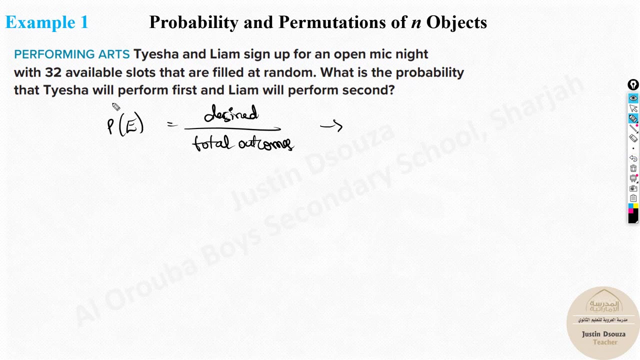 perform second. now here, what is the desired possibility we want? we want taisha to perform first and liam to perform second, and there are total 32 available slots out of 32. the first one must be taisha and second one itself must be liam. how many possibilities can this happen? 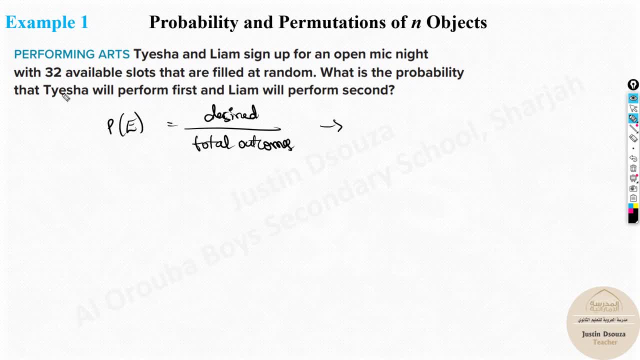 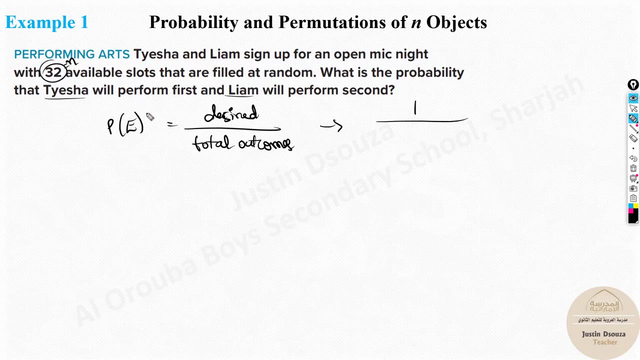 there's only one possibility. it's like you know: taisha must be first, liam must be second. this, this is just one possible way that can occur right, so desired over here is one. what is the n value? the total availability is n, that is 32.. r is the selection over here. 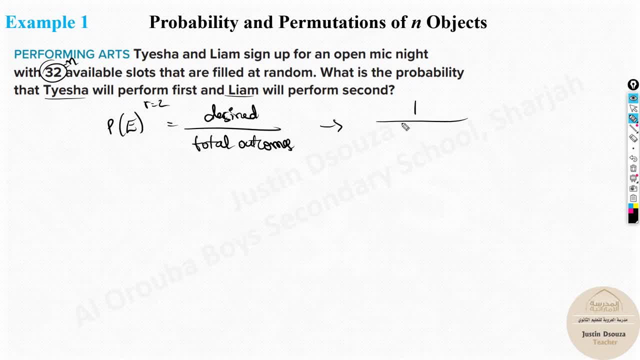 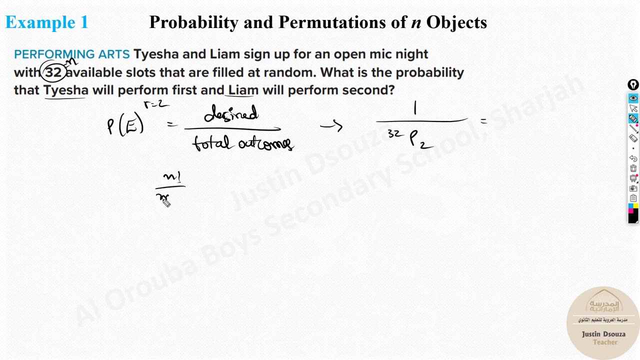 taisha and liam. there are only two people, so r will be equal to two. so now over here, the total outcome will be n, that is 32 p 2. this is the answer. now here, you can solve by using the formula that is n factorial by n minus r whole factorial. 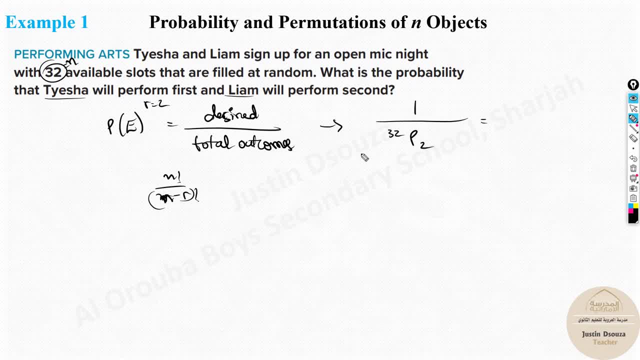 now this factorial. everything can be solved in calculator. now, if you know this formula, you can just write it some way, and then you can directly use the calculator and solve it. what i would suggest is So what you can do is you can just write: NPR equals this formula some way. 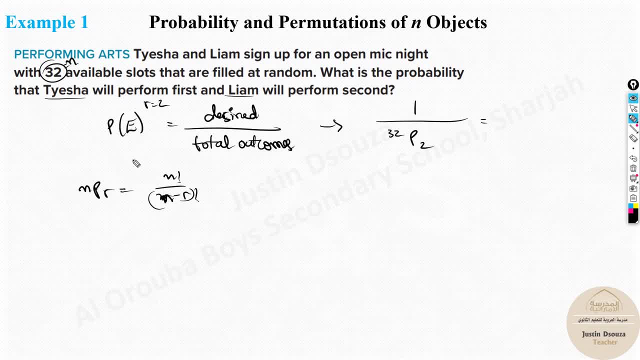 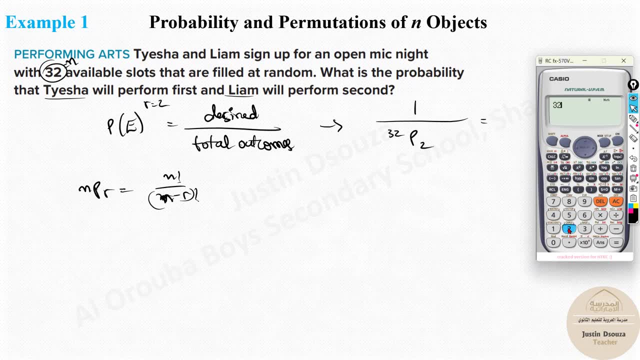 And no need of using it. If you know the formula, it's more than enough. You can just directly, you know, put it in the calculator which I'll show you now. Now I will solve this individually. first, 32, where is P? 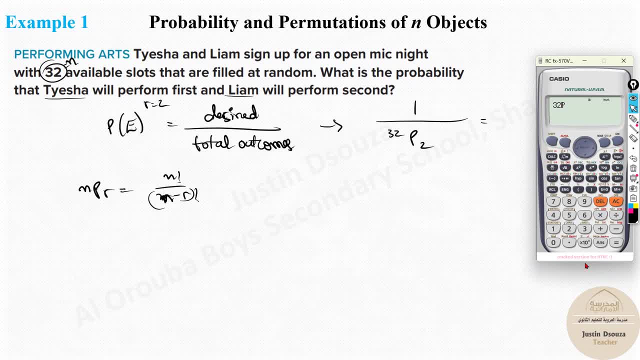 P is by shift and this over here: multiplication symbol, That's the P value, If it is C, it's shift, and division symbol, And R is 2.. This is the total possibilities. But here we have 1 divided by right. 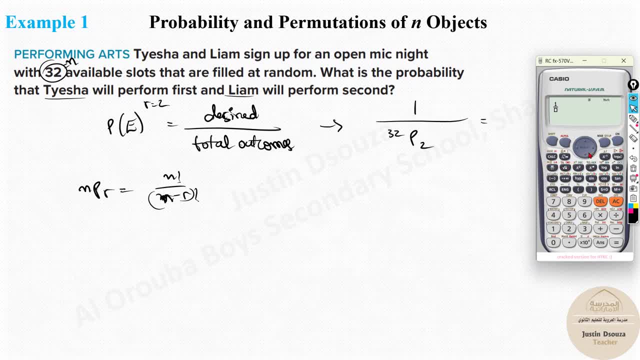 So you can just write it like this: 1 divided by 992 was what we got, But let me just write it 32P2.. I wrote C. Sorry, that's wrong, It's P2.. It's 1 by 992.. 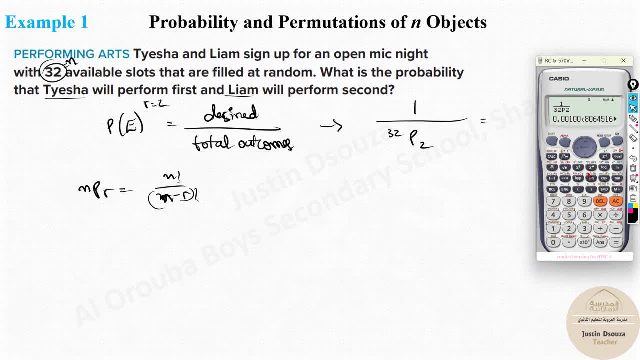 That is the probability. It's 0.001.. If you want the percentage, you just multiply this by 100. You will get the percentage over here. Just multiply by 100. That's the percentage. It's like 0.1%. 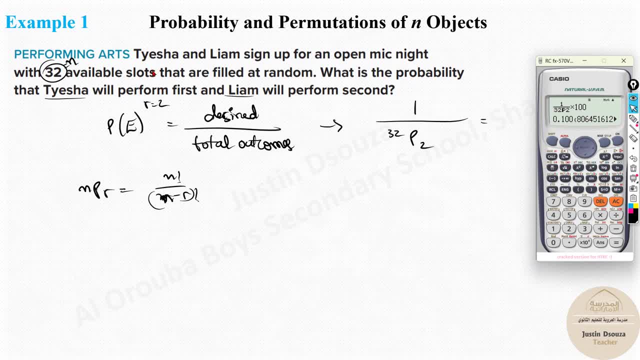 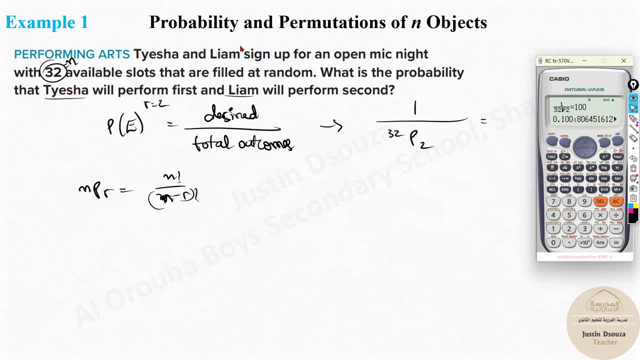 0.1%, That might happen. Okay, Always, when you get the answer, try to relate and understand the given situation And you can, you know, understand whether it's true or false. So this is the answer. You can write it in fractions itself: 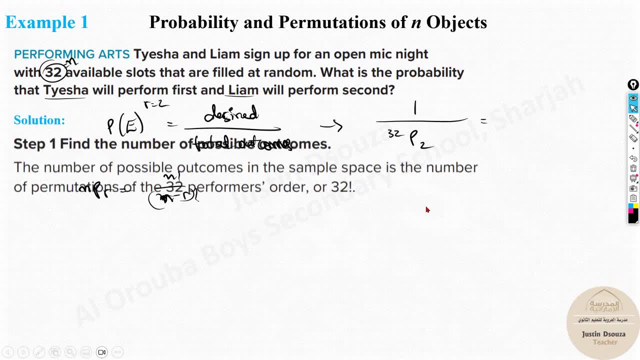 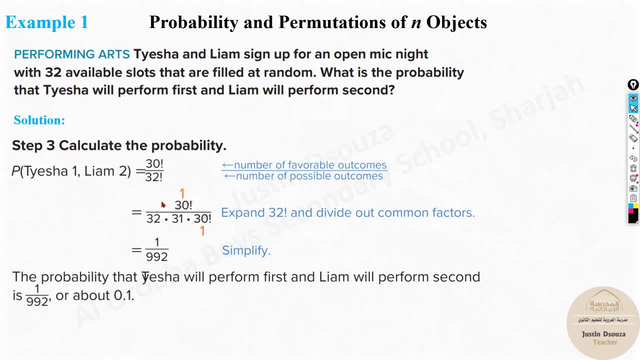 Sorry, I'll just remove it. It's 1 by 992.. Let's over here. They have used some other method. I guess That's fine. The final answer will be the same: Why I told you, this method is designed by total outcomes. 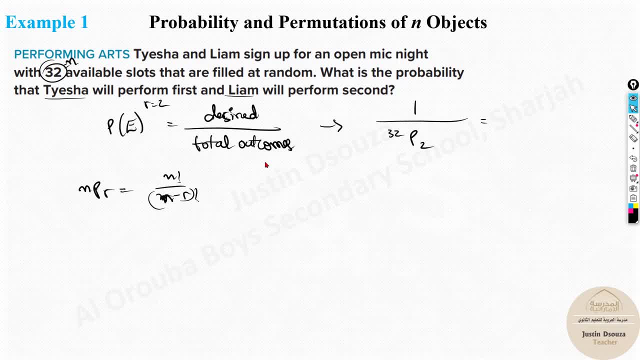 Because whatever you saw over here can be used all the time and you will definitely get the correct answer all the time. So just stick to one probability method every time. If it's for combination, it's just the formula that changes. Now we will look over here. 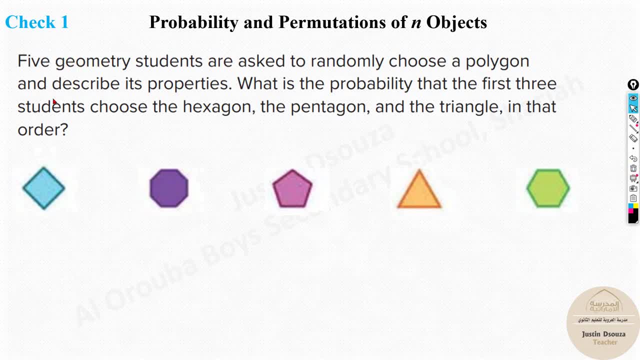 Five geometry students are asked to randomly choose a polygon and describe its properties. What is the probability that the first three students choose hexagon, the pentagon and triangle in that order? See, now, It's very important. There is an order over here. 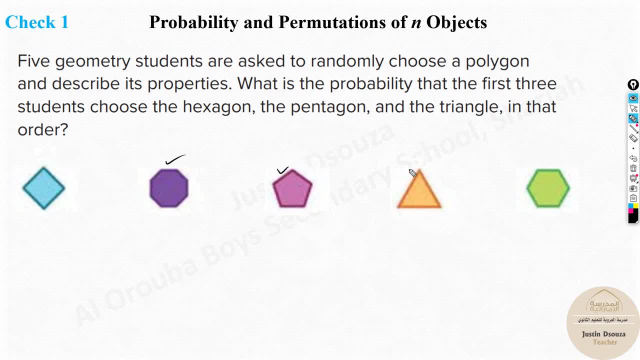 Hexagon is chosen first, pentagon next and then the triangle. no matter what, All the three students must choose the same order. Order is important. It's a permutation problem. We can understand it easily, But now what's the answer? 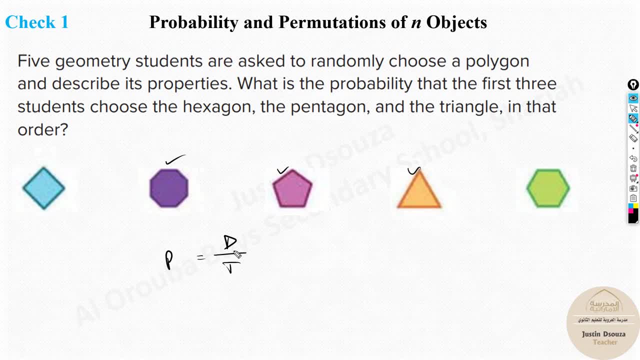 Probability would be equal to. I'll write: desired by total. This D is for desire, desire divided by total. Now, what is the desired? Hexagon, pentagon, triangle. all must be in order, right, It's only one possibility, one desired outcome, because there is no more. 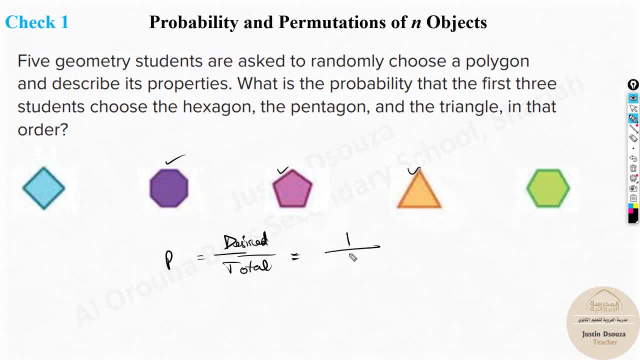 Only. this is the exact way to select, So it's only one possibility, divided by Now, what is happening? There are five geometric figures right. There are: N is phi, P, R is the selection? How much is the selection that's made? 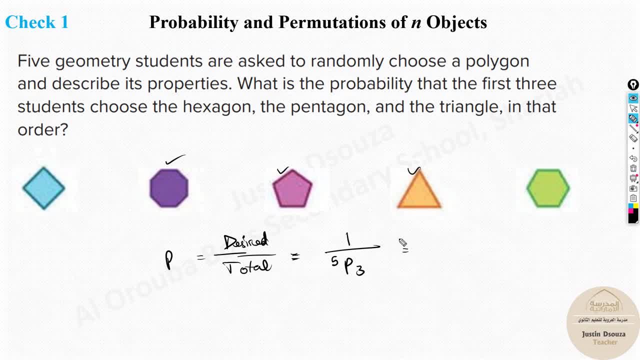 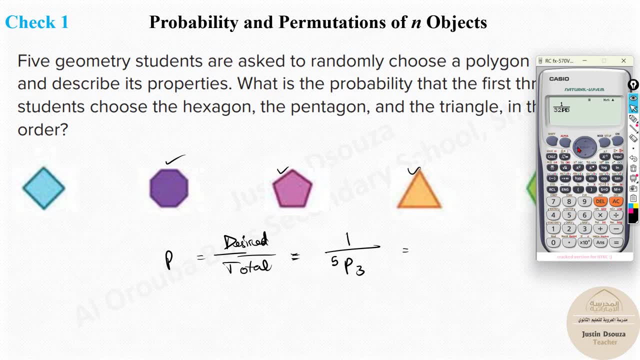 One, two, three. So it's phi, Phi, P, three. So you just put this in the calculator, You should get the answer. I'll use the same one, Just change R to three and N to phi. here The answer must be one by 60, and that's it. 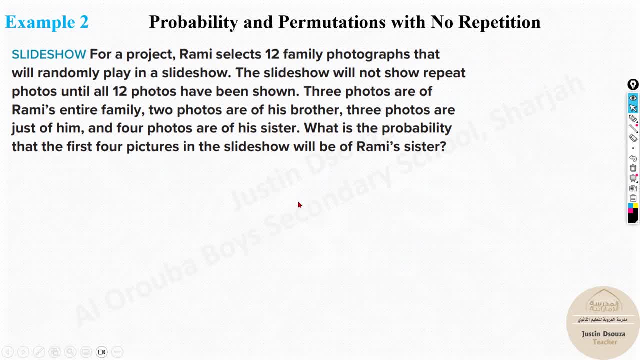 So this is how we can easily solve it up. Now let's look into another problem here. For a project, Rami selects 12 family photographs which will randomly play in a slideshow. The slideshow will not show. It will repeat photos until all 12 photos have been shown. 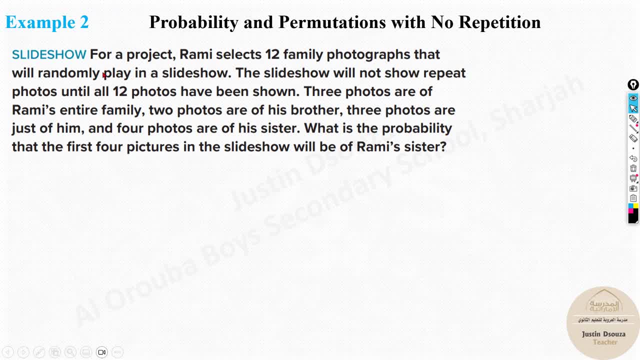 That means each order is important. after one, the other, one other one and so on. Three photos are of Rami's entire family, Two are of his brother, three are of just him and four photos are of his sister. What is the probability that the first four pictures in the slideshow will be Rami's sister? 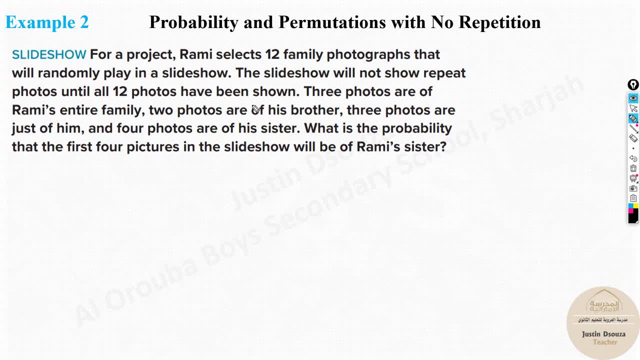 So now here. first thing, what is N? Let's note down a few things. That N is 12.. This is not R. This is saying: how many photos are there? Three photos are of his family, two are of his brother, three are of him, four are of his sister. 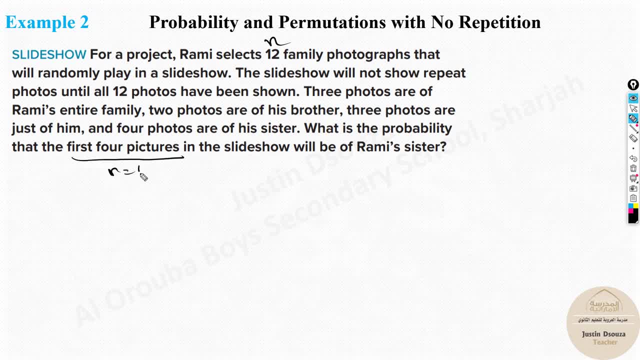 What is the probability that the first four photos, R is four here. This is the selection. What do you want? Okay, R only of Rami's sister. Now here there is an important thing to remember: In the previous problems it was only one possibility, divided by the permutation. 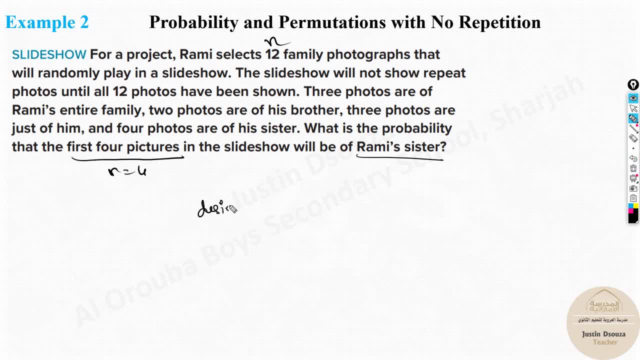 Right Here. it's not like that Desired by total right. This is the probability. probability of any event. What is the desire over here? It's his sister's photos. How many photos are there? There are four photos. 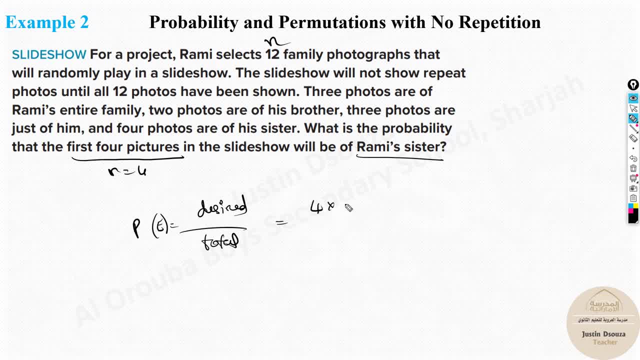 So the first possibility is: out of four, any one can be chosen. Then, once one is chosen, how many more possibilities are there? Three possibilities, Then again there is two possibilities And lastly there is one possibility because there are four photos of sister, of his sister. 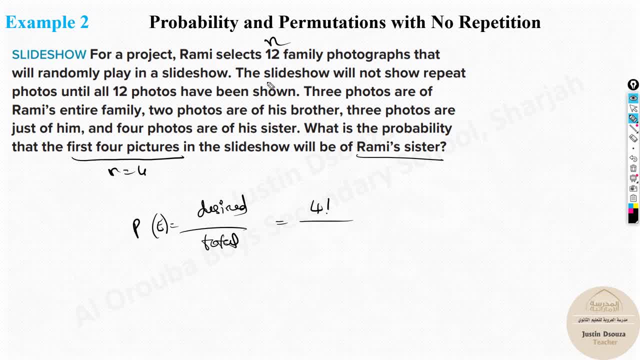 So you can directly write it as four factorial. What is the total? N is 12, P, R is four. So I'll just change this into 12 over here. So one more thing when you're solving it directly, right? 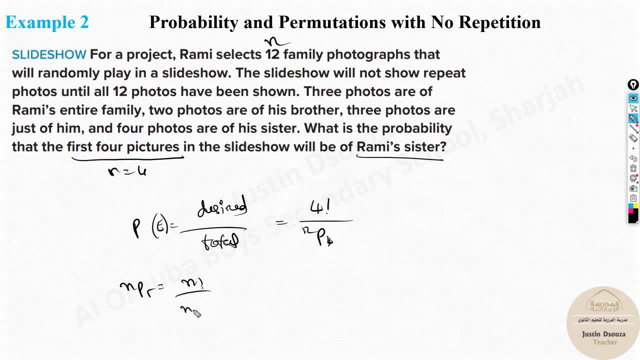 What is NPR, N factorial by N minus R, the whole factorial. That means you know the formula. You can use the calculator itself to solve this formula. So just write it out. But now we will directly use the calculator and solve it. 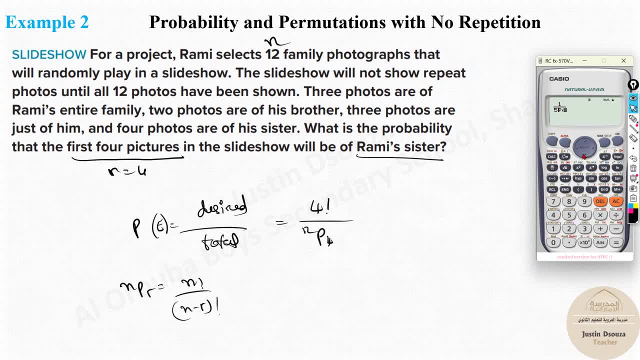 I'll just change this up. over here It's four selections, That is, R is four and N is 12, the total number of photographs And what is the desired one. over here It's four. factorial. Now, where do you find factorial is Shift and the symbol. 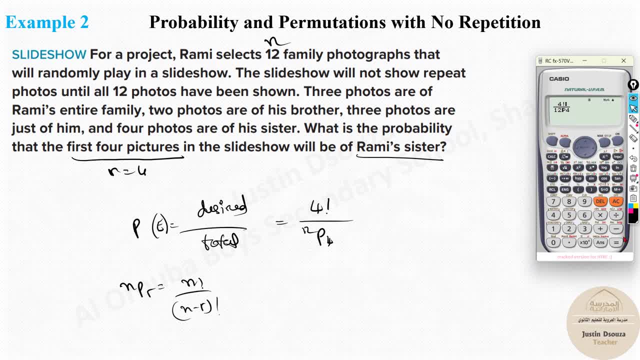 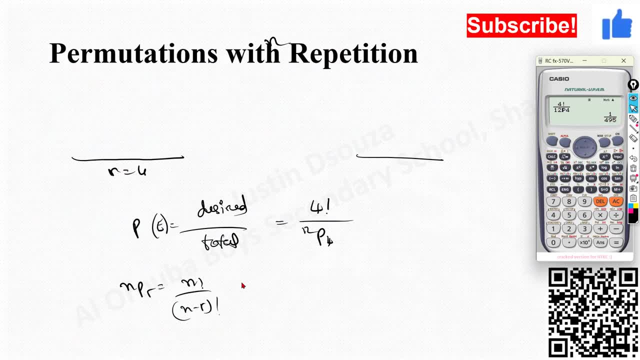 It's above the X inverse. That's by shift and X inverse symbol. We'll use you it now. It's for 1 by 495.. That should be the answer And we? yeah, that was the answer. I guess it's 1 by 495.. 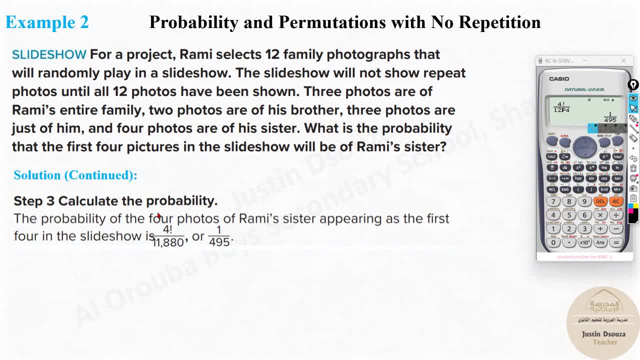 Now here, the total possibilities are 11,880.. Yes, but we are, you know, having four factors in the numerator, So it becomes 1 by 495.. Now, if they just ask you what is the total possibilities, 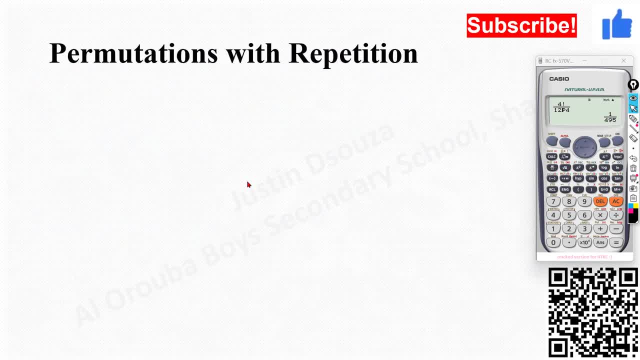 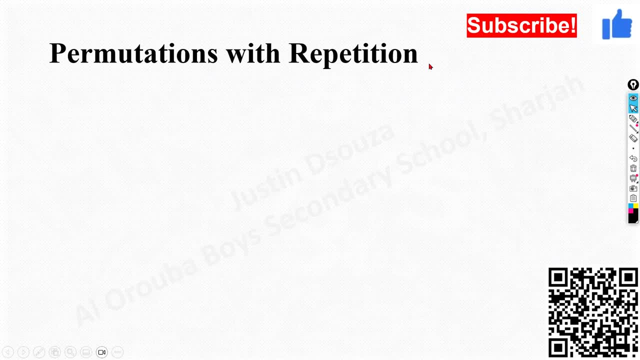 This is the answer. 12, P 4.. That's it, And now we will see Another important type of problem, That is, permutations with the repetition. Before I continue, a quick reminder: please do consider subscribing to my channel, If you have subscribed to it. 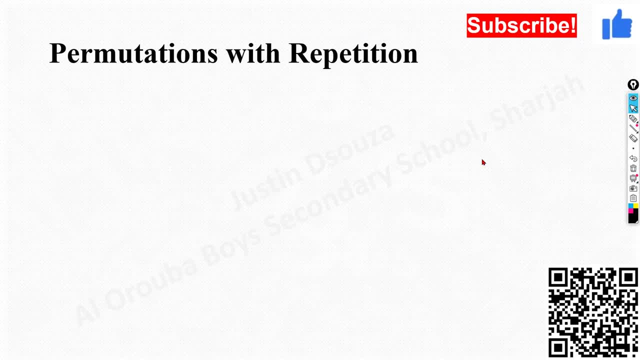 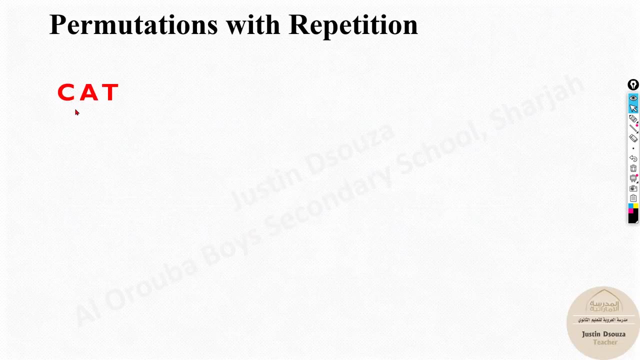 Thank you so much And please do like and share my videos. I would love it so much. Thank you, guys. This is another interesting topic: permutations with the repetition. Now, imagine we will just go to our example and then we will see what exactly repetition would mean. 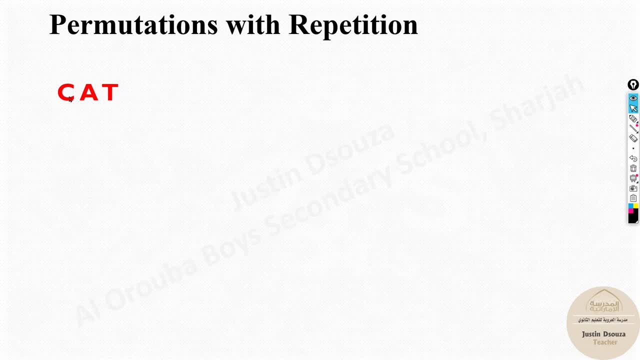 Imagine you have the word Cat. How many different ways you can arrange it. It's basically three factorial right, Because there's three possibilities. So it's either CAT, CTA, or then now take A is the first letter, then ACT or ATC. 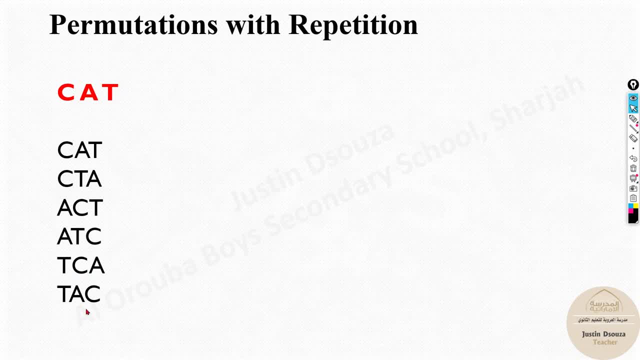 And then lastly, TETCA or TAC. This is six. Now what about the letter MOM? Because there are three letters. It should be three factorial, isn't it? But now, let's try it, It'll be MOM. 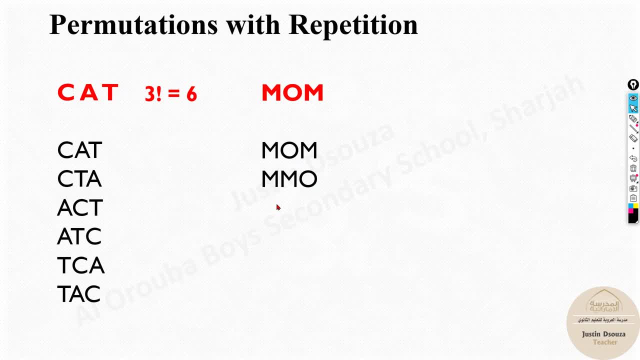 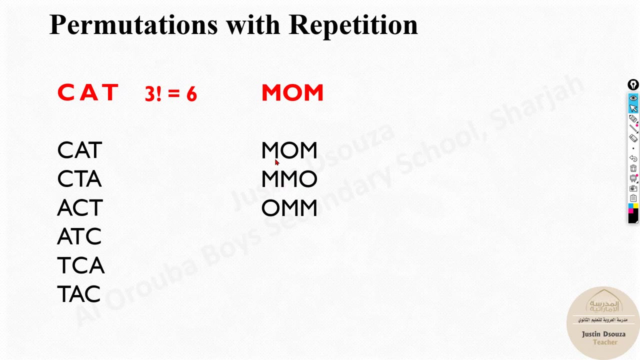 I will write MMO or I'll bring this O to the first, and now doesn't matter what I do. These are both the same letters, M, So doesn't matter I flip this. It's the same thing, isn't it? M and M. even if I swap them, they'll be the same thing. 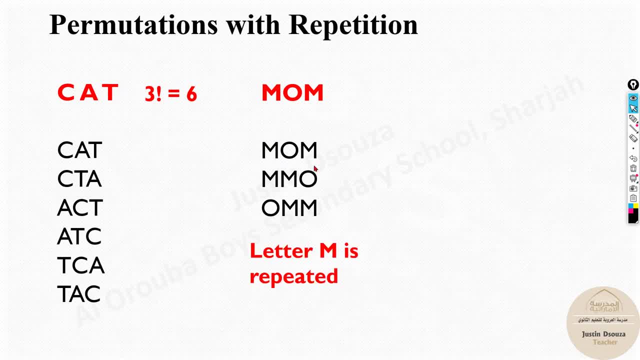 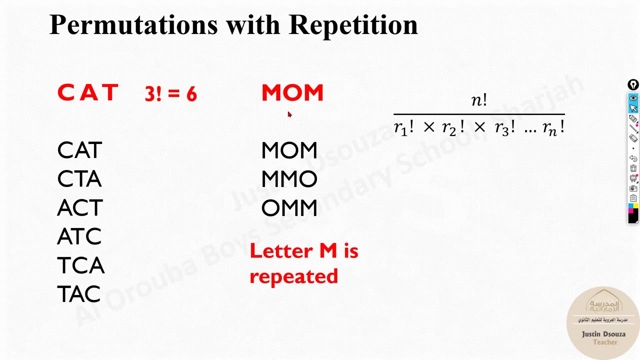 So here the numbers are repeated. So how many possibilities? Only three possibilities. How do we know? So the formula is very simple: Total number, that is n, factorial. That is what we do for general problems If there is no repetition, but if it's repeated, divided by the number of repeated letter. 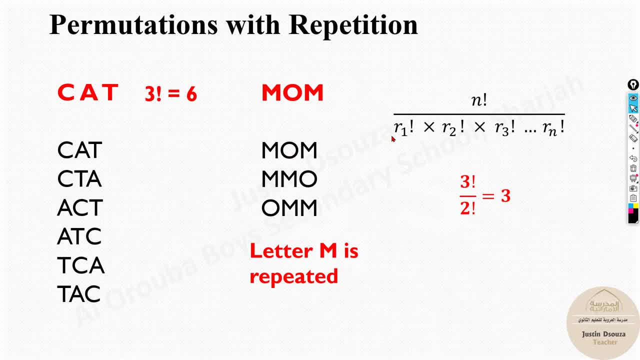 What is it over here? M is repeated. How many times? The number of times it's repeated? Sorry, it's three. factorial by two: factorial, That is three. That's the answer. Now any other letter, count the number of repeated alphabets and then solve it up. 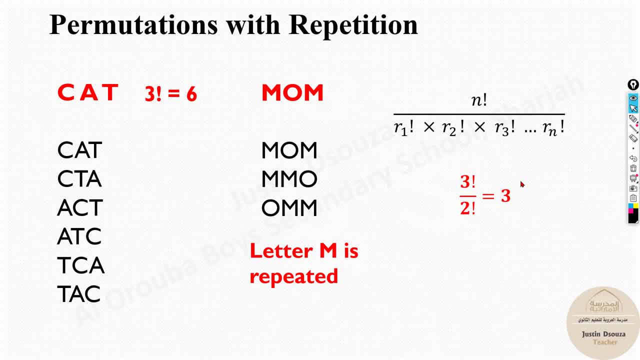 Here one more thing: Please avoid using NPR formula. There is, there is cases where you can use and solve it, but it's just complicated, So I will tell you the easiest method. So just avoid NPR formula when it comes to repetition. Now let's look at this problem. 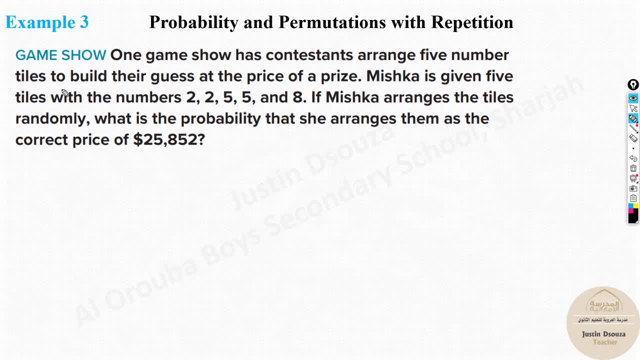 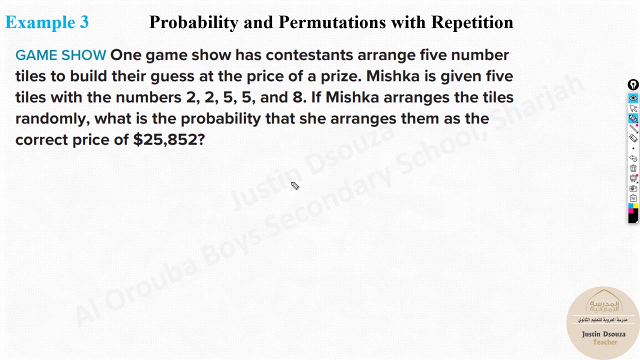 One game show has contestants arrange five number tiles to build their guess at the price of a prize. Mishka is given five tiles with the number zero, Sorry, 22558.. If Mishka arranges the tiles randomly, what is the probability that she arranges them as correct? prize of 25852?. 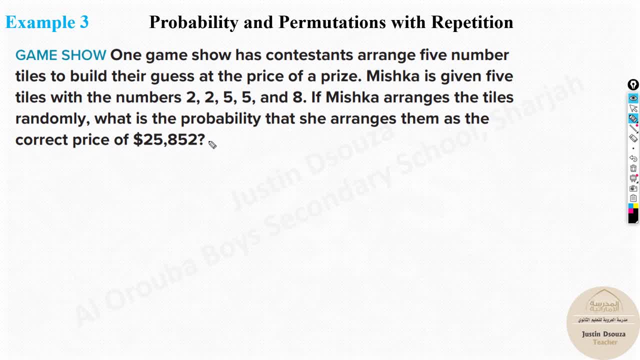 So this is the exact number, This is the price that must be arranged. Now. what are the possible ways that this number is exactly arranged? What is the probability or what is the chance? Yeah, how many total numbers are there? One, two, three, four, five? factorial. 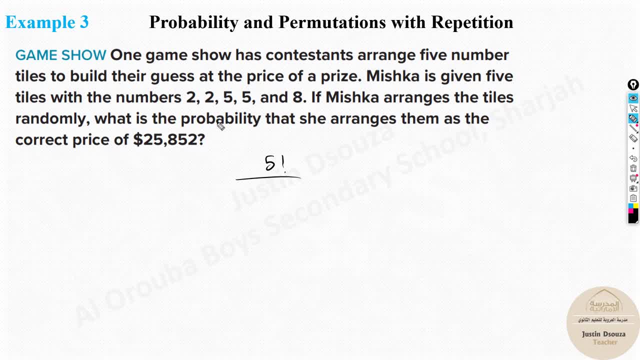 Right. But what happens? Two is repeated two times, So two factorial. It's not because of this number. How many times is it repeated? If it was another two, two to two, I should have written three factorial here. The two is repeated twice. 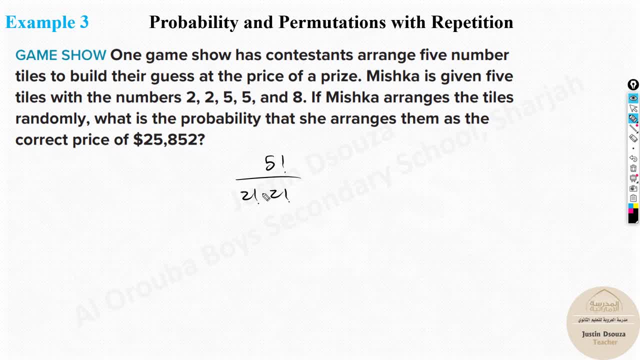 And what about five? again repeated twice. So it's five factorial by two, by two factorial. So this is the answer, This is the total possibilities, that that these numbers can be arranged to the correct number. Now, the correct number is only one possibility. 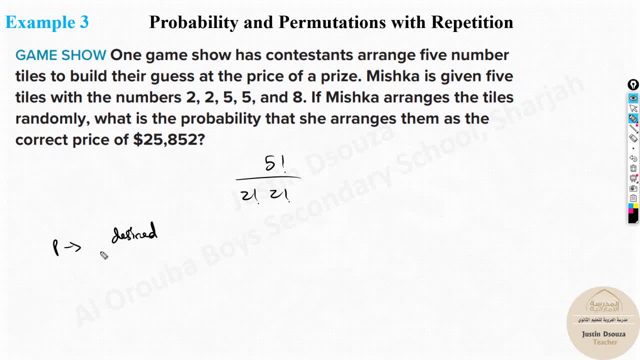 Probability is always desired by total, Isn't it? Now, what is the desired over here? This is desired by total. desired is only one, because this should be the exact number. That is the desired. So it's only one possibility and total is basically over here. 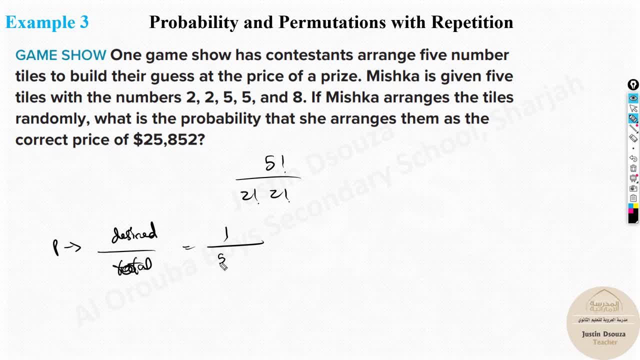 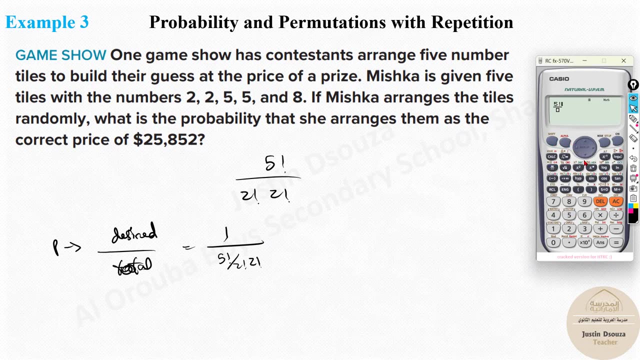 Whatever the answer you get, Okay, it's well, just write it over here: Five factorial divided by two factorial into two factorial. You can put this everything in the calculator directly and get the answer As well. But what I'll do is I just find this probability, this five factorial divided by two factorial- 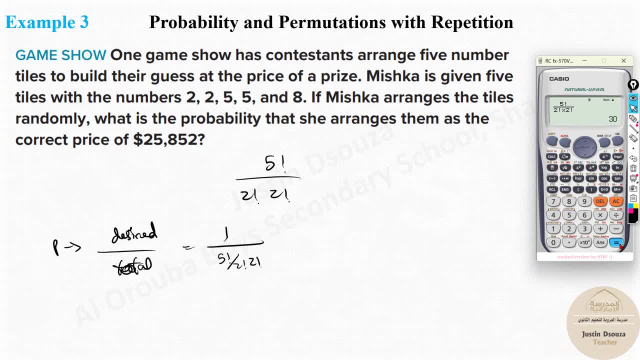 Into two. also, You can do or just write it to factorial itself. for this one The answer is 30. So it is 1 by 30. There is a chance of 1 by 30 times that this actual number can be guessed out. 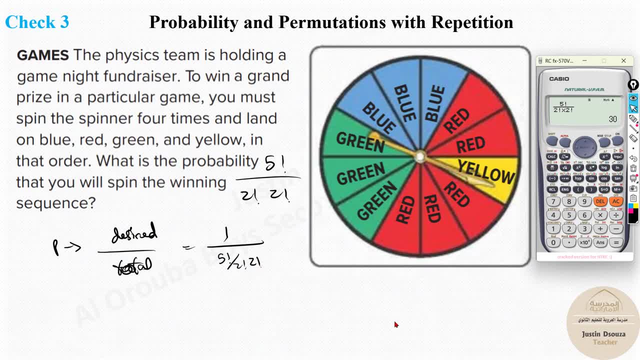 Okay, so the answer is 1 over 30.. Let's look at another. The physics team is holding a game night fundraiser. to win a grand prize in a particular game, You must spin the spinner four times and land on blue, red, green and yellow, in that order. 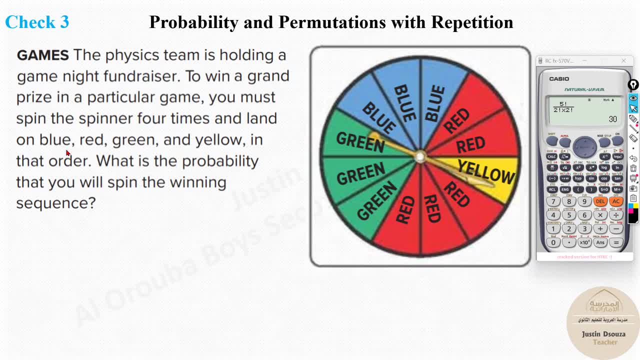 See, this order is very important. Blue, red, green, yellow. order gives out that it's permutation. What is the probability that the spin that you will spin the winning sequence? Now we are. how many possibilities are there in total? Let's count. 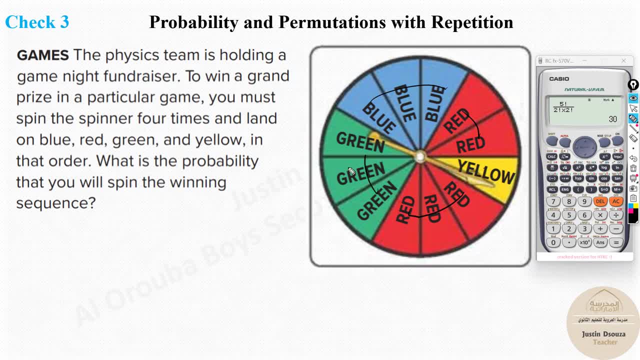 There are three Blues, Three, four, five, six, One, eight, nine, ten, eleven, twelve, So n is basically two. earlier The total, Let me write 12, factorial. But what is repeating here? One, two, three. 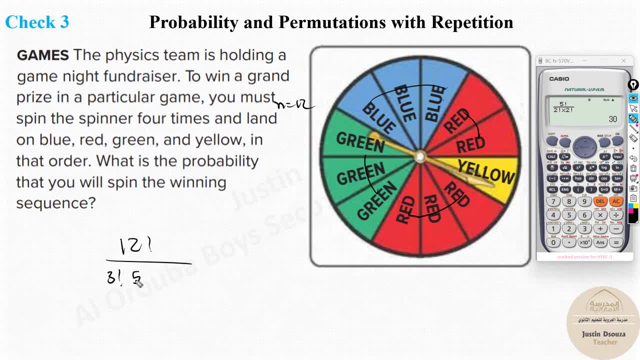 Blue is repeated, three factorial. What about red? Five factorial. Why? Because one, two, three, four, five. And what about the green? Again, three factorial. So this is the total possibilities, And now, if you want to put the winning sequence, it should be blue, red, green, yellow. 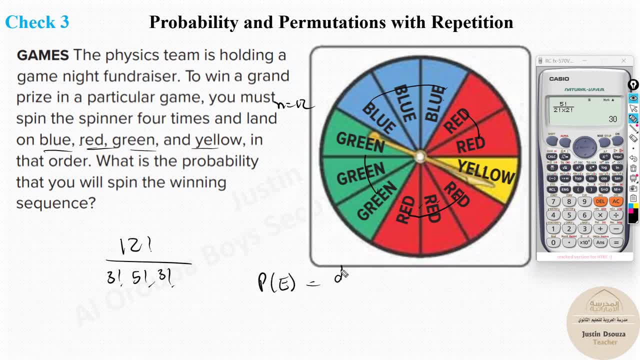 It's only one possibility, isn't it? Probability of event is desired by total. So here the desired. What is desired exactly? It's only one divided by whatever this answer you get here- Let me just change it up- instead of five. 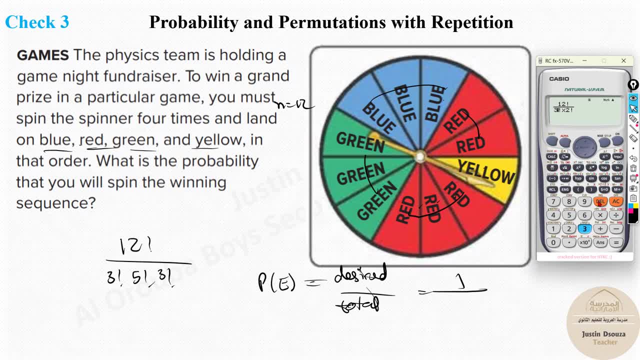 We have 12 factorial divided by three factorial multiplied by five factorial And again last we have three factorial shift and inverse. So it's one by eleven hundred and ten thousand Eight hundred and eighty. So this would be the answer. It is one, one zero, eight, eight zero. 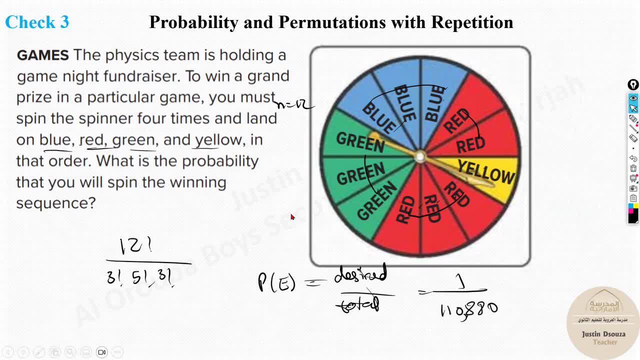 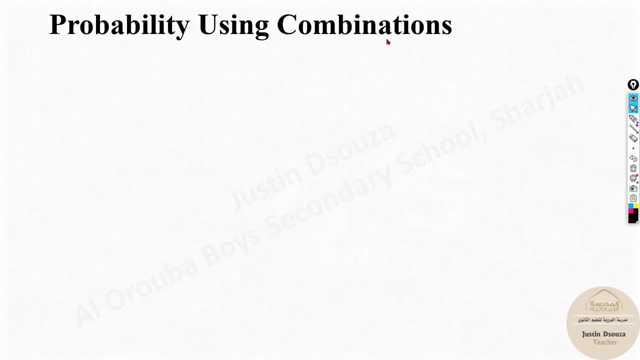 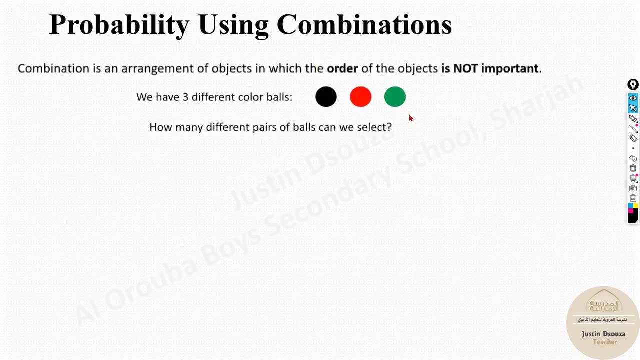 So it's hundred and ten thousand eight hundred and eighty, So it's a very, very rare scenario. That's how we solve this particular problem. Now we go to probabilities, using combinations. This is another interesting one. Here the order is not important. 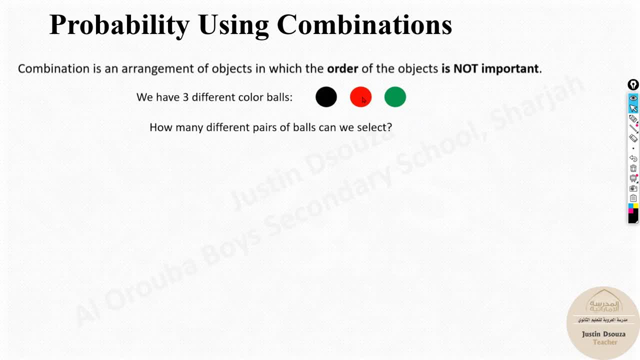 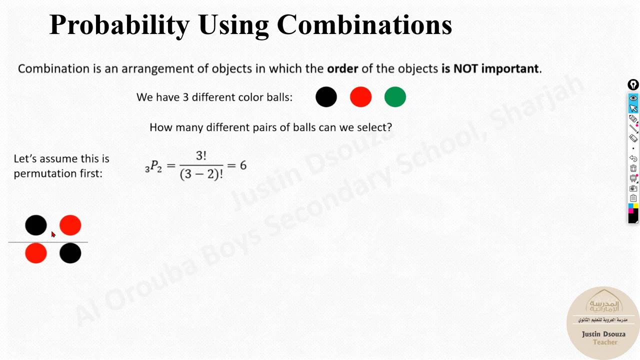 If the order is not important, Imagine you need to select these Three balls just like how we did in permutations. Now let's do with combination. Select them here without any order. So one way: see over here if it's a red, black, red or red black. 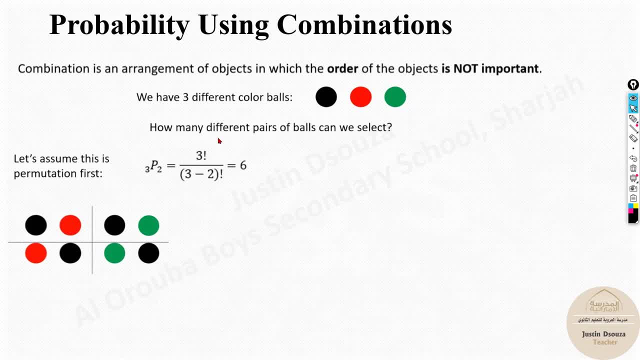 It's the same thing. It doesn't matter here. This was for the permutation. Sorry, We used to see the order is very important and it was six possibilities for permutation- Just now we saw this. but now for combination, it doesn't matter. 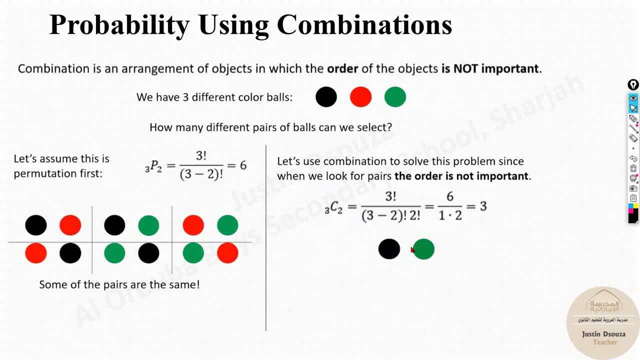 This is the same thing. One possibility Is red and green, or even if it is green or red, It's fine, It's the same thing. or it can be red and black, or red and green, That's it. These are only three possibilities, because you're in whether it's black or red, or red and black. 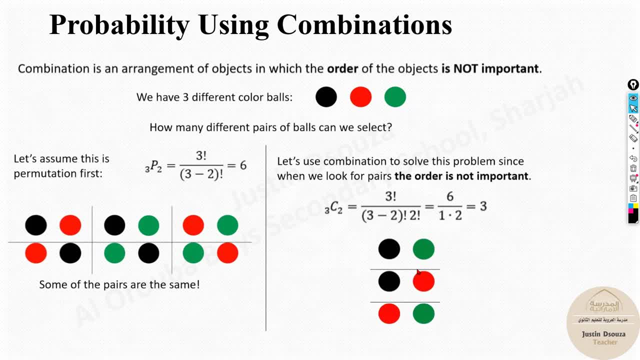 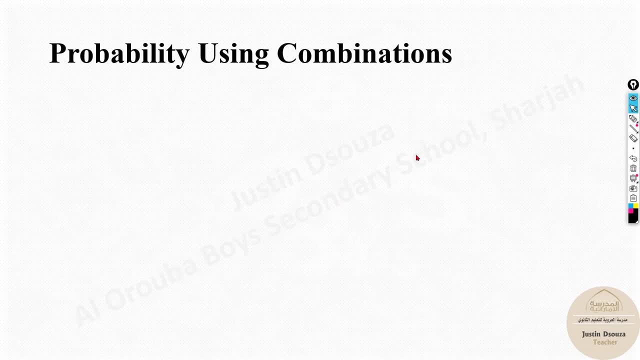 It's considered the same thing after all. They're the same balls, right? You're just arranging the position of the order, which is not important in combination. So that's the thing. the probability using combinations is given by NCR. It is not P over here. 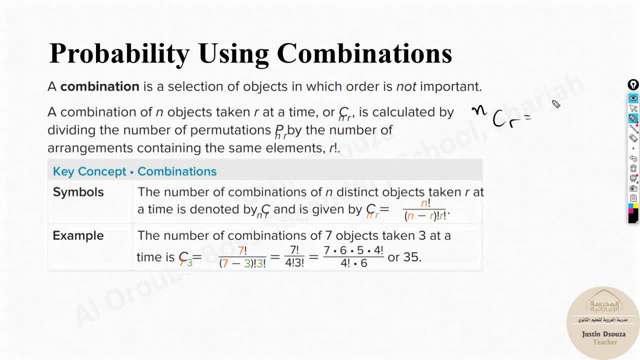 Permutation is P and CR. This formula is given by N factorial, by R factorial, into N minus R, the whole factorial. or sometimes you can write it like this also, It's the same thing what I've written: NCR is equal to N factorial. 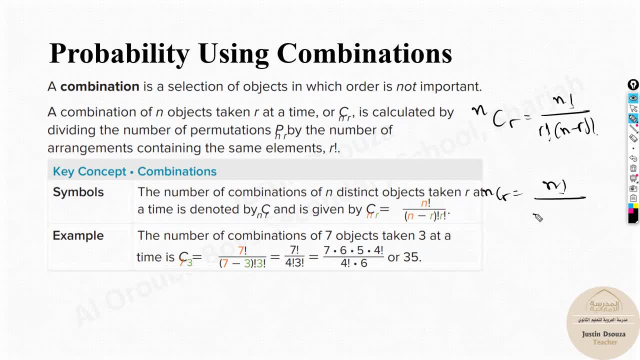 I've just written R first. I usually write R first, but it's fine. N minus R, the whole factorial into R factorial. It's the same thing Again. you can directly solve this in calculator. but please do mention this, mention this formula, and then what you can do is: you can directly solve in calculator. 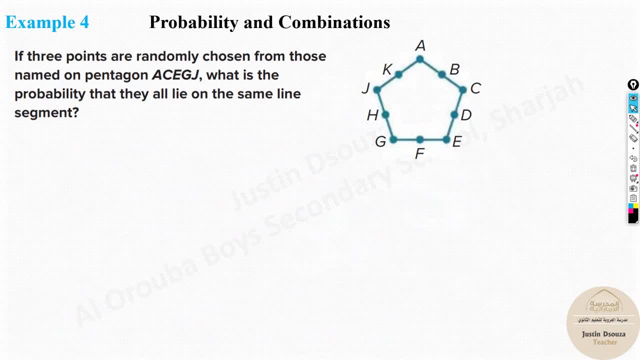 We have an interesting problem here on combinations. If three points are randomly chosen from those named on Pentagon- A, C, E, G, J- What is the probability that they all lie on the same line segment? Let's count the total number of points. 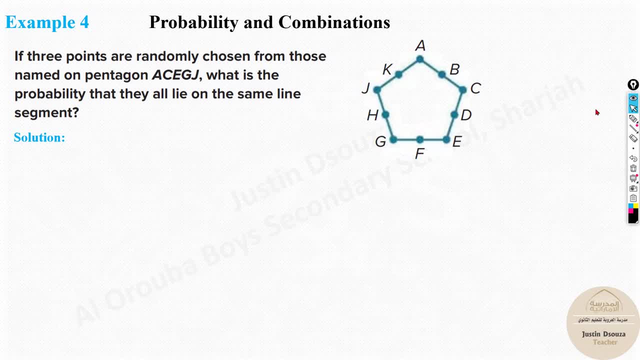 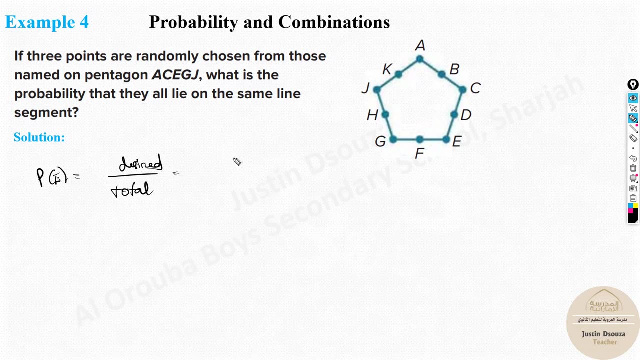 How many it is. 3,, 6,, 9,, 10 points are there, So N is 10.. Now, before that, again, probability of any event is given by desired, by the total So desired and total over here Desired. will come to it in a while. 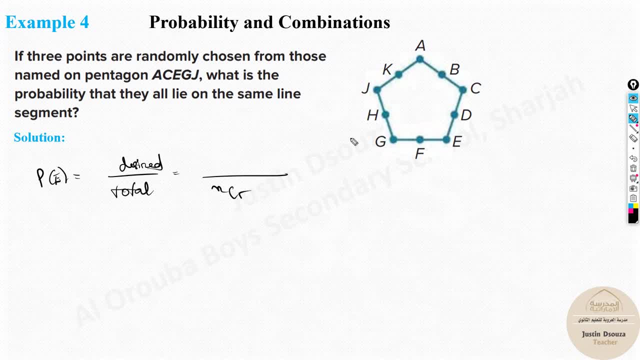 This total is given by NCR, isn't it, This NCR? What is the N value over here? We just now counted: N is 10 C And what are the? you know what is the selection? Three points are randomly chosen. 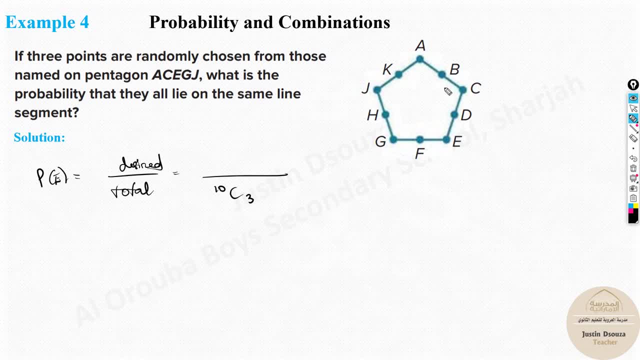 So the selection is three. That's it Here. It's given three points are randomly chosen. Now what is the desired outcome? What is the probability that they will all lie on the same line segment? That means the three chosen points can be JKA. 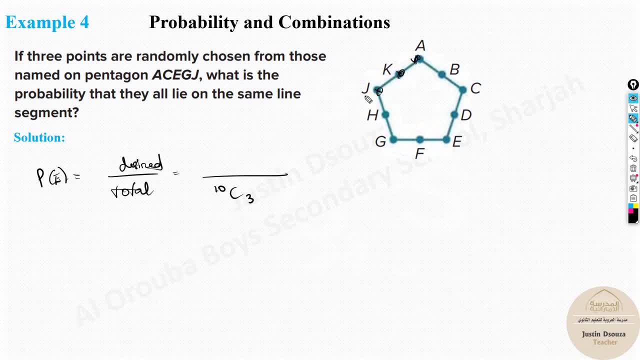 Okay, doesn't matter the order, It can be a k, you know, a kj or kaj or anything. Or then another possibility is ABC, or another one is CDE or DEC or C, You know any. any order is fine. 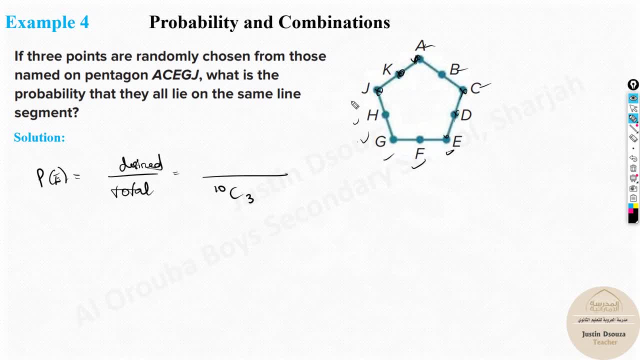 And then we have EFG, And lastly again we have GHA. So how many lines are there? One, two, three, four, five. So there is totally five possibilities. Now let's write the formula for NCR. 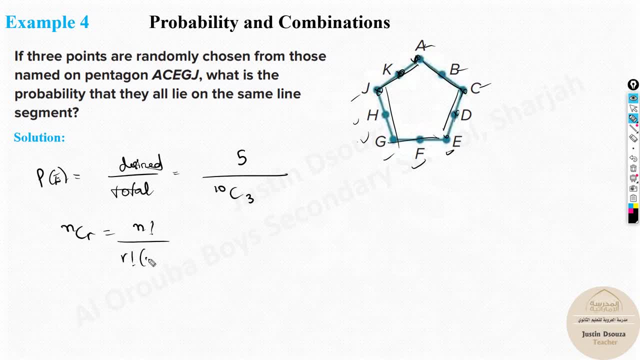 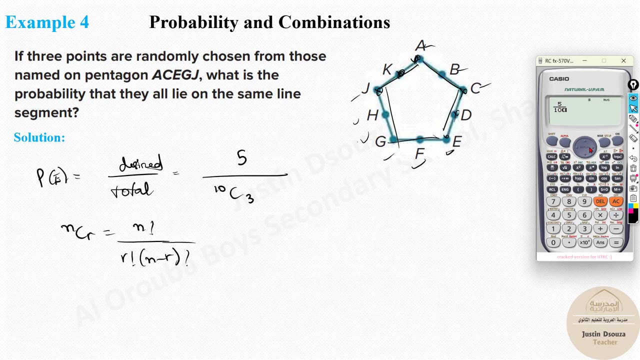 It is given by N factorial divided by R factorial into N minus R, The whole factorial. Or you can write N minus R factorial into R factorial. We will solve it up in the calculator directly: 5 divided by 10.. C is over here, shift and division symbol, and R is 3.. 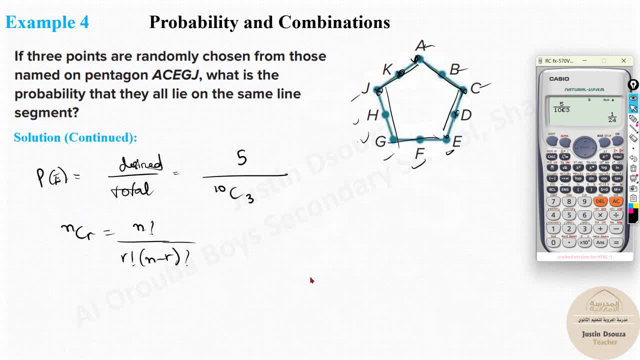 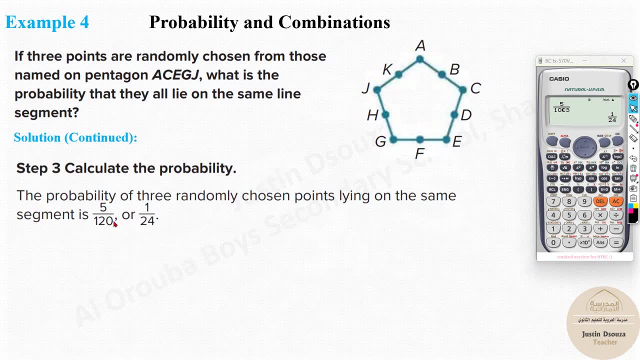 The answer is 1 by 24.. So here you can see, the final answer is 1 by 24.. If you do 10C3, it is 120 possibilities. But now here we have five desired outcomes, So it will be 1 by 24.. 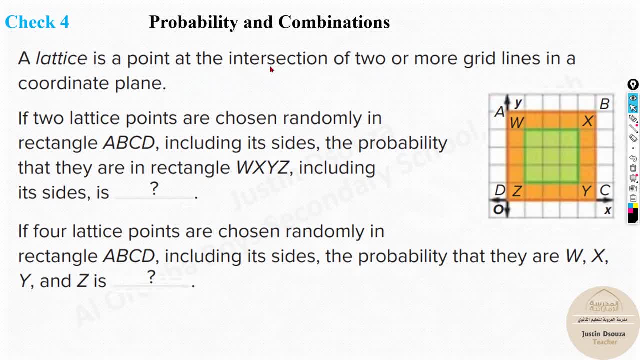 The last problem in this lesson. It's about a lattice. Lattice is a point at the intersection of two or more grid lines. You can see over here, whenever grid lines intersect, That is a lattice point. over here, All these are lattice points. 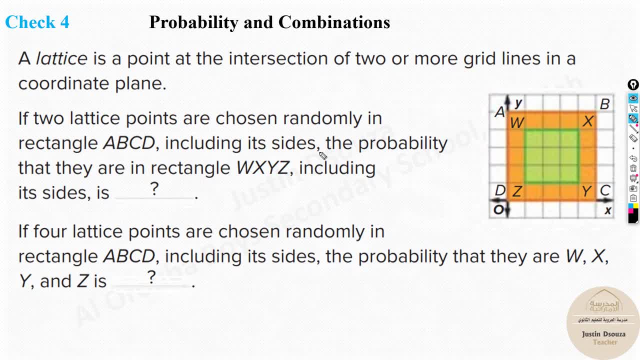 Okay, if two lattice points are chosen randomly in rectangle ABCD- See ABCD, the outer rectangle, the orange color one- Now orange color is Entirely this entire thing- Okay, whereas WXYZ is only the green one. Now two are being chosen randomly in the triangle, rectangle ABCD, including its sides. 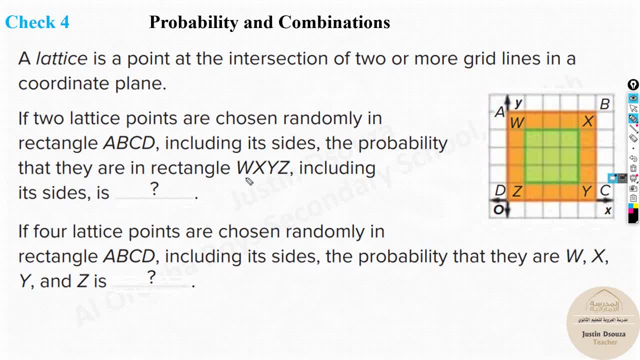 The probability they are in rectangle WXYZ, including its sides, is Now here. you're just choosing two random points in within this triangle. Okay, any two random points, But what is the probability that they fall within this triangle, Within this rectangle? it's all squares over here, but still square is a rectangle itself. 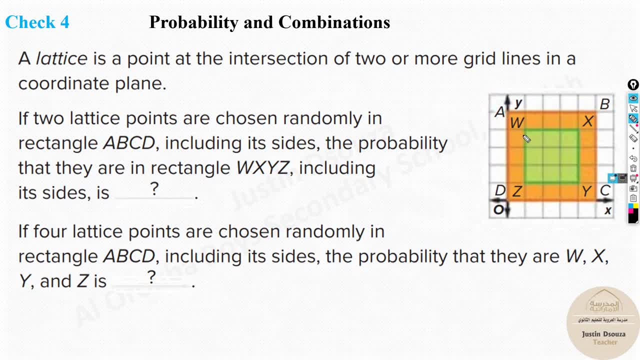 So they're just mentioning rectangle. It's fine. Now what is the desired iron total? So in such problems, right, You can use NCR, but NCR, NPR, But what I would personally do is- since it's countable over here, 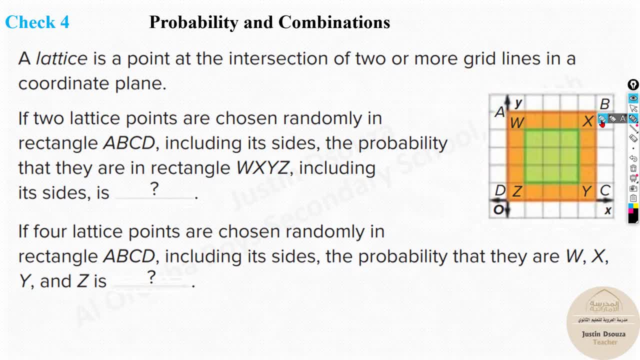 You can just start counting it Now, when you have such graph, such problems, where lattice points are to be considered, What is the total lattice points? You can count the sides and sides and multiply, but I will just mark out all the points to make it easy. 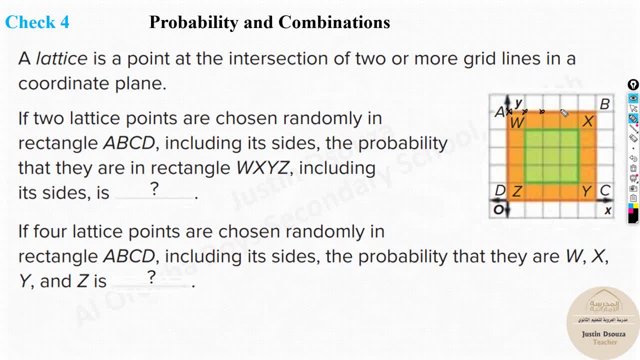 So what is the point of your one? This is a lattice- point 2, 3, 4, 5, 6.. And again over here: 7, 8, 9, 10, 11, 12, and it goes on, so you can do one side and one more side, 3, 6.. 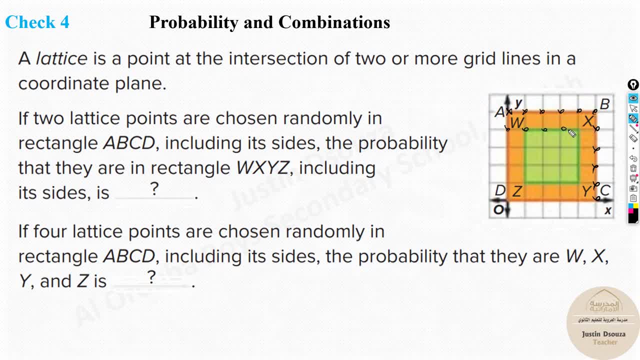 So 6 times 6 would be 36.. Or you can just count them All. count them All, you will get 36.. See, these are all for the triangle rectangle ABCD. So these are all the lattice points, isn't it? 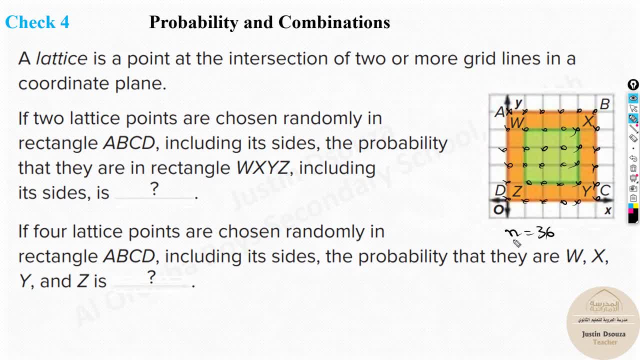 So that is n. n is equal to 36.. What is the selection? selection is our R is how many two lattice points are being selected, that is 2.. Now let's write the probability formula. probability is given by desired divided by Total. and what is desired over here? 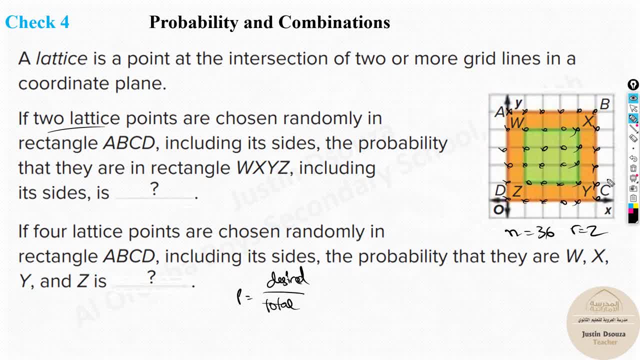 Now, again, we need to count them because desired is within this rectangle. How many are there within the rectangle WXYZ, the inner rectangle? Let's again count it. This would be 1, 2, 3, 4, 5, 6, 4 and 4.. 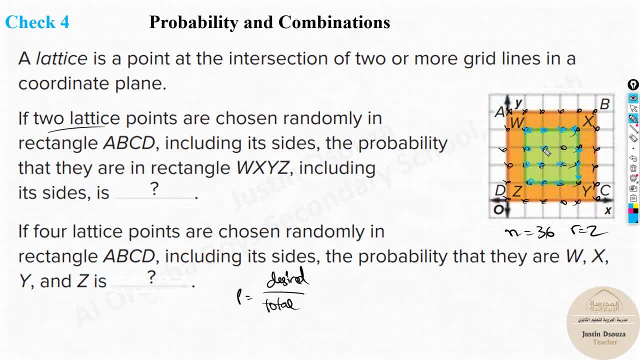 It will be 16.. Okay, if you. these are the ones, the ones in blue. Now for ABCD, all are included. Okay, Now desired would be 4.. 4's are 16.. Now, here again, Remember 16.. 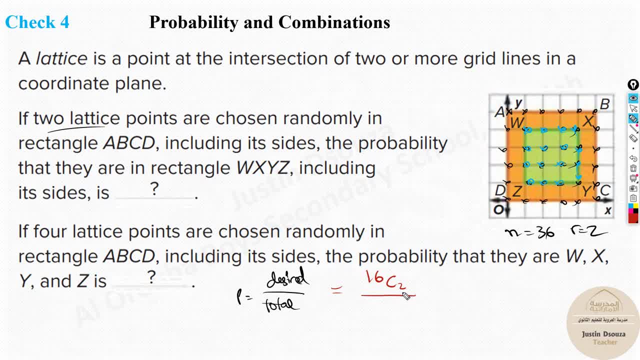 What is it Just 16.. No, it is 16 C2.. Why? because all these are possible. right 2 are being selected. either this or this or this, there are various possibilities. So all 16 C2 over here. 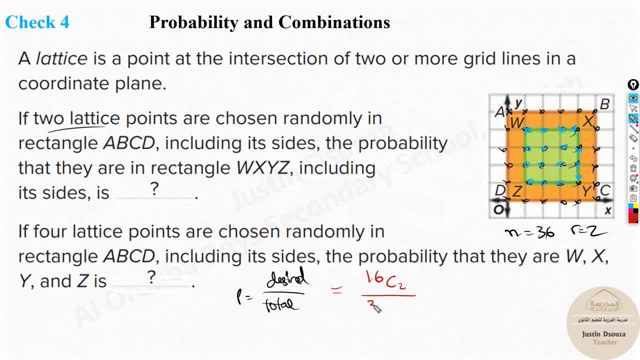 Also, you need to use combination. and what is the total? total is basically 36 is n. We have got C2. just put this in calculator. You will get the first answer. And now what about the next one? Let's write it and then I'll use the calculator together. 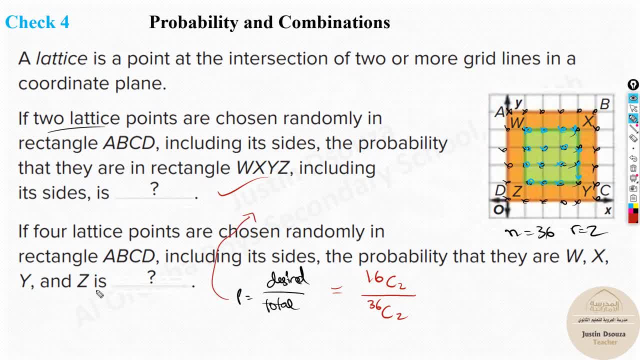 This was supposed to be written up. Okay, this is over here. and the next one. probability would be desired by total if four lattice points are chosen randomly in the rectangle ABCD. So again, for the total, the n is same- 36- only the R value changes. 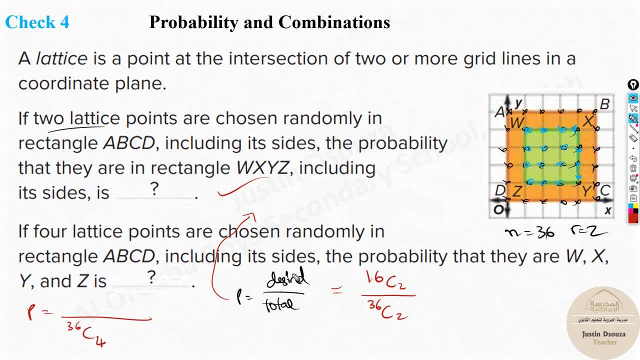 How much is R? R is 4, this time Including its sides. Yes, the probability that they are W, X, Y, Z. So now they are telling what is the probability that will be W or X or Y or Z. So these, what is the problem? that they will be these four particular points. 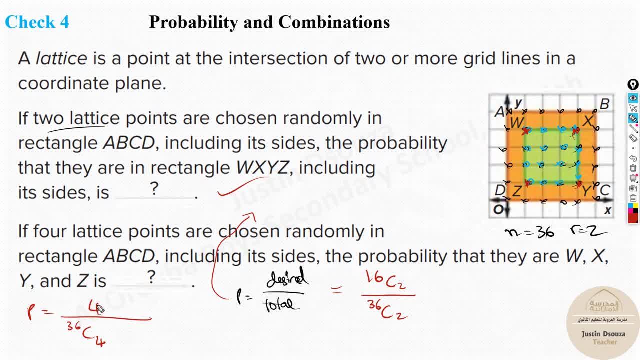 It's only four possibilities, right? Sorry, I'm wrong. Four are being selected. They must be, for it is basically one possibility, Okay, one Possibility. but if you're thinking okay, I will write in terms of NCR. 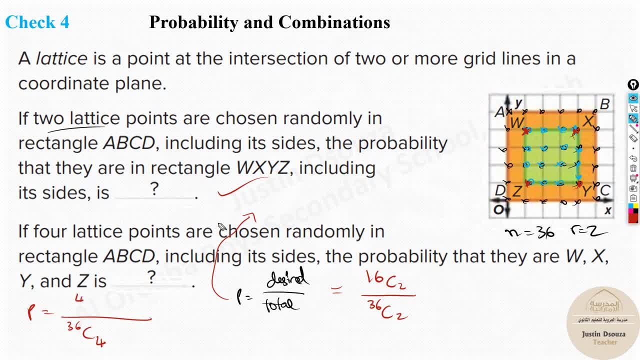 Okay, Yes, you can do. there are four points over here, possible points, and you're selecting for 4 C. 4 is 1, basically, Okay, this is the way to write. I've written 4 C 4 Y, because I've written this as to write. 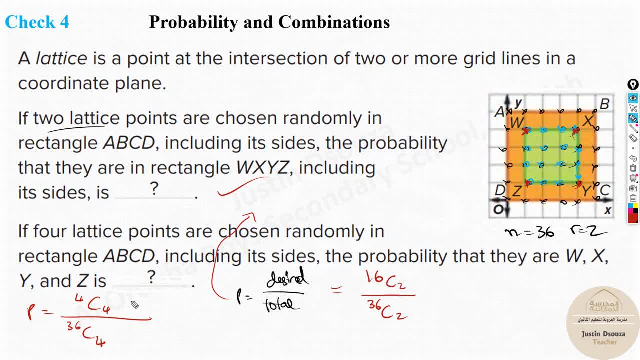 So that's the reason we are also have written 16 C, 2. That's the reason. all you can easily understand. W, X, Y, Z, 4 points also have to be selected. Only one possible way, that is, one over here in the desired outcome. 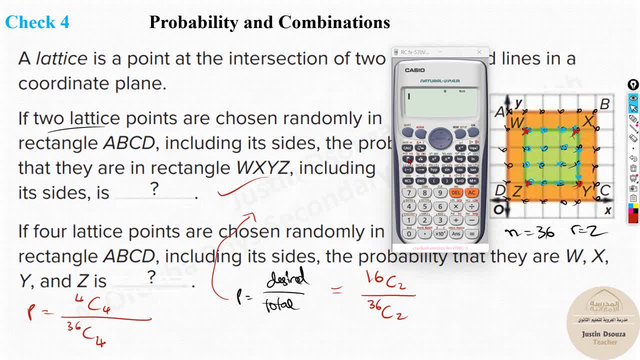 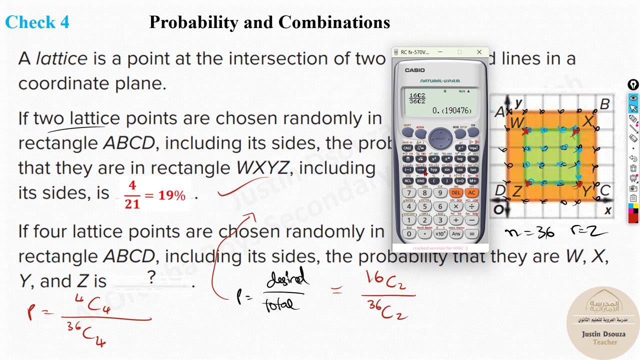 So now we can just put this in the calculator and solve it up. The first one is 16, C is by shift, and C 2 divided by 36, shift C 2. The answer must be 4 by 21.. Yes, and you can find the percentage by multiplying by hundred. over here will be decimal, will go to the other side, will be 19%. 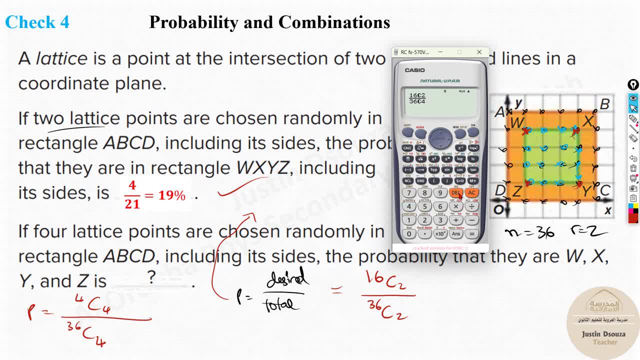 Now the next answer would be over here, for, and even over here, It will be 4 C, 4 or 1.. You can write it: It is 1 by 500 and 558 thousand nine hundred and five, or if you do it as person, it will be 0 point. 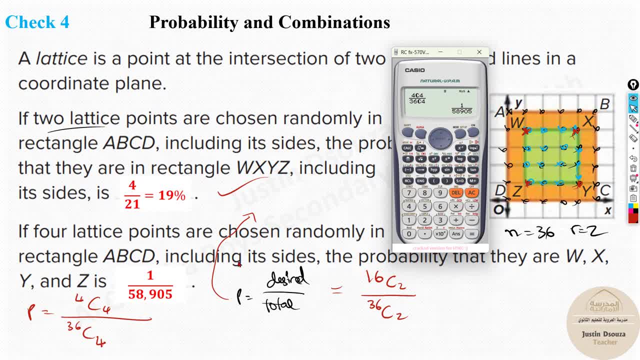 It's negligible, So just keep it as fraction itself, because the- you know it's such a huge number- will be 0.00. so on, Right. So this is the answer: 58.. One thousand nine hundred and five. I hope this is clear.